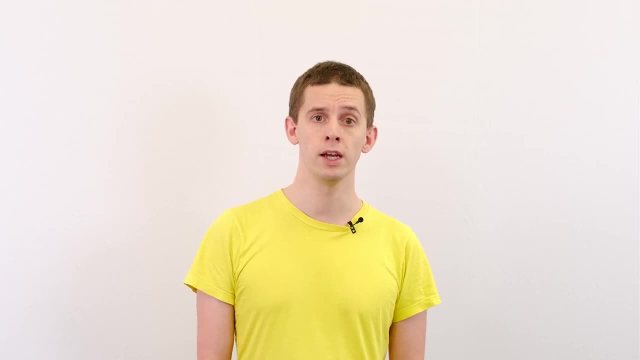 features of the SVD and is one way that we can get a lot of insight into a matrix's structure. It's also useful for effectively compressing the amount of information that is stored in a matrix. One of the most useful properties of the Singular Value Decomposition is that it allows us to 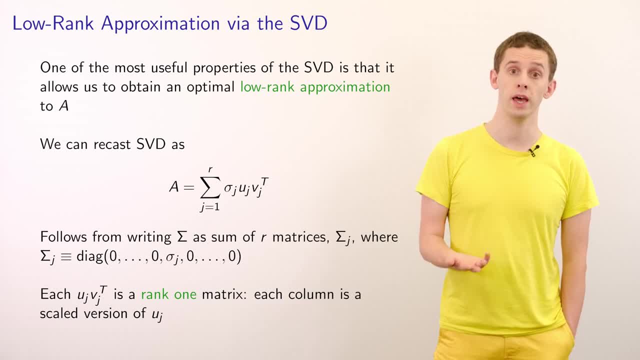 compute an optimal low-rank approximation of a matrix A of size n by n, And to do this we can recast the Singular Value Decomposition, referred to as the SVD, in the following form: We say that A is equal to the sum from j equal 1 to r of sigma j times uj, times vj transpose: 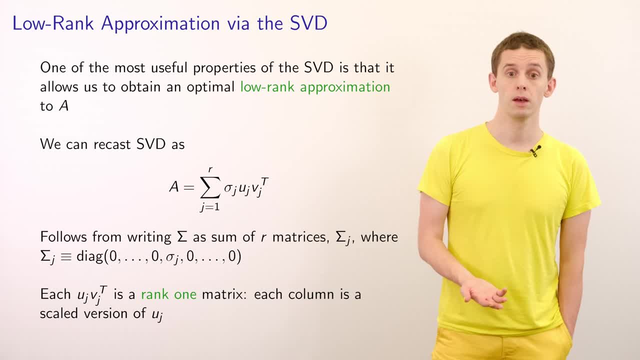 where r is the rank of our matrix A And this follows from writing our matrix sigma in terms of the sum of matrices. sigma j, where sigma j is defined as a diagonal matrix but where only the j-th singular value is present in the j-th row and j-th column. 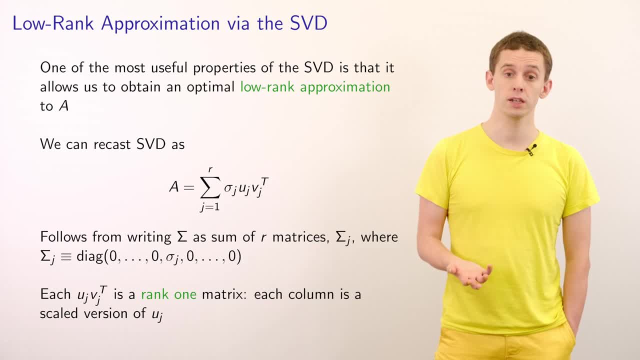 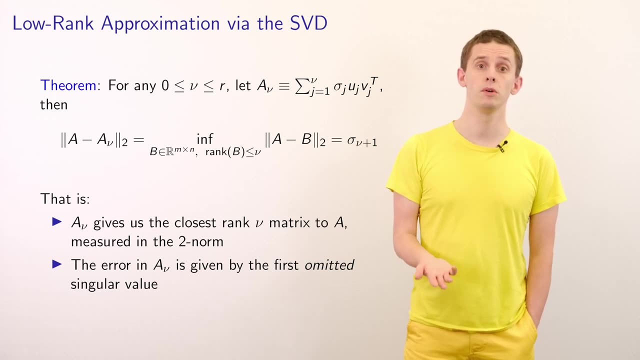 If we look at each factor uj times vj transpose, then we'll see that this is a rank 1 matrix and each column is a scaled version of uj. Suppose that nu is between 0 and r and let's define A subscript, nu, to be the sum from j. 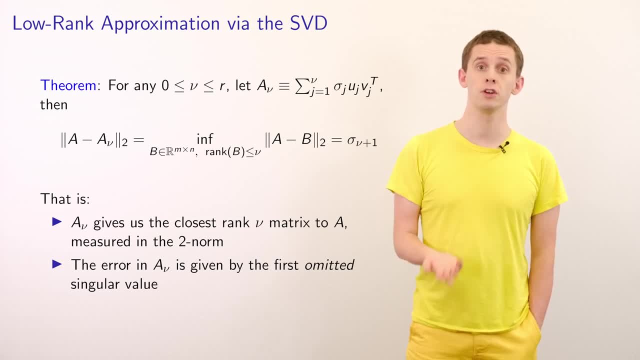 equal 1 to nu of sigma j times uj times vj transpose. So in other words, we take our full sum, that would go from j equal 1 to r, and we truncate it after just nu terms. So we have the following theorem in this case: 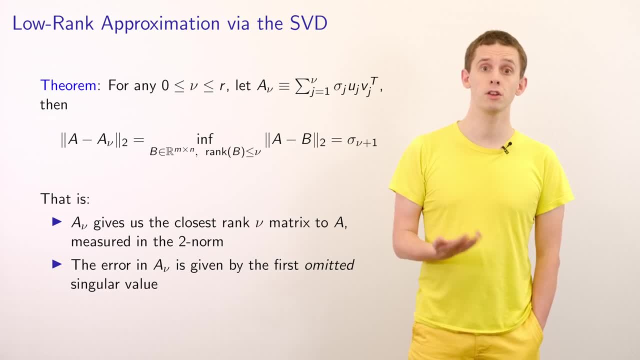 Suppose that we look over all matrices B Of rank 1 to r, Of rank less than or equal to nu, Then we find that the difference between A and B in the induced Euclidean 2 norm will be minimized when B is equal to A subscript nu. 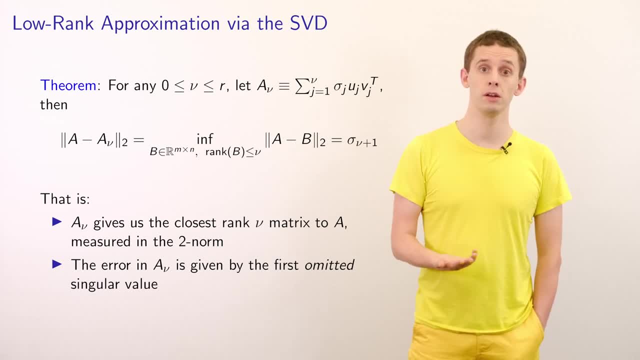 And furthermore the value of that induced Euclidean norm difference will be equal to sigma nu plus 1, ie the first singular value in the sum that we neglected. So in other words, A subscript nu gives us the closest rank nu matrix to A measured in.